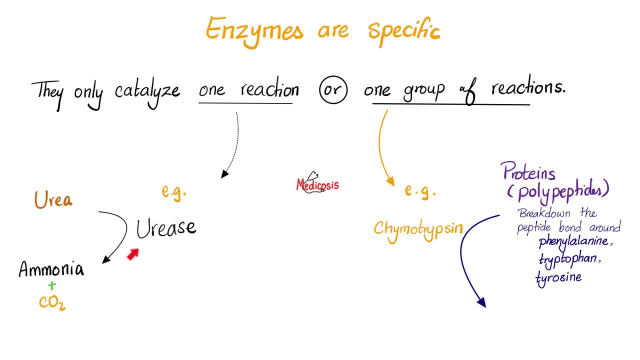 medicine. later you will learn about some bacteria that are urease positive, ie they possess the enzyme urease, such as the famous helicobacter pylori, which can lead to peptic ulcer disease. How about enzymes that are specific to one group of reactions? This is chymotrypsin. Chymotrypsin. 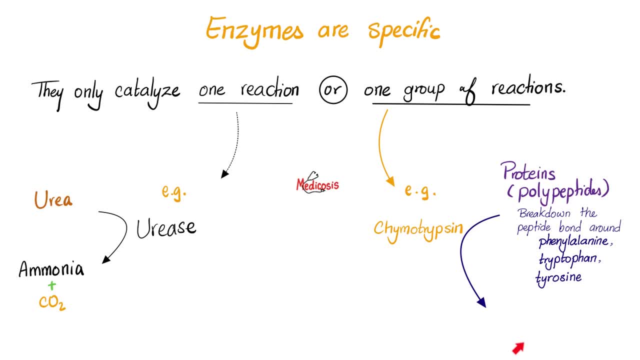 can break down proteins or polypeptides by breaking down peptide. Chymotrypsin can break down peptide. Peptide bonds around phenylalanine, tryptophan or tyrosine, So it's not just one thing. 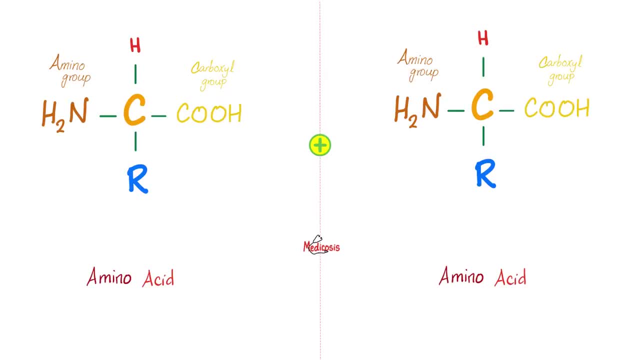 It's a group of things within the same category. Do you remember when we talked about the peptide bond before? All right, let's try to make a peptide bond. Okay, we're trying to join two amino acids together And you make a lovely peptide bond between them. And, of course, 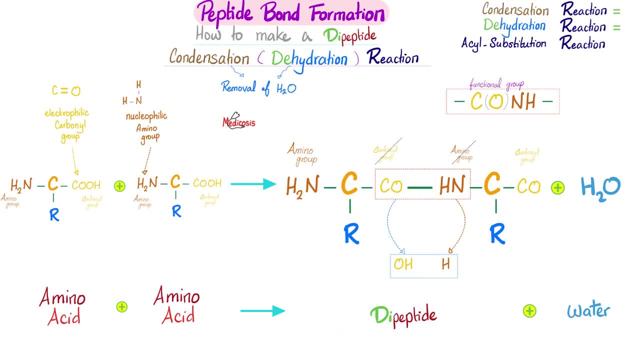 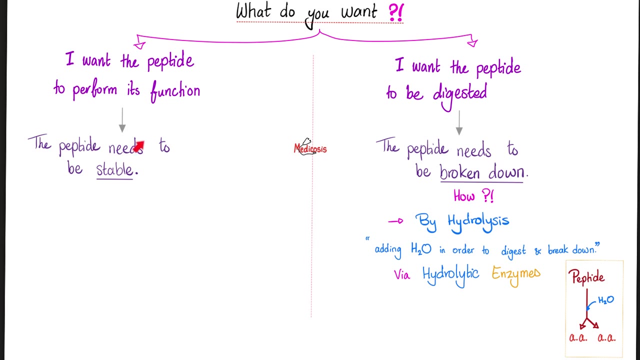 WOTA has left the chat. This was an amino acid, This was another amino acid, But now you have a and WOTA. And what's that? A peptide bond. It depends on what you're trying to do. If you're trying to make the peptide function, you need to make the bond stable. If you want it to be, 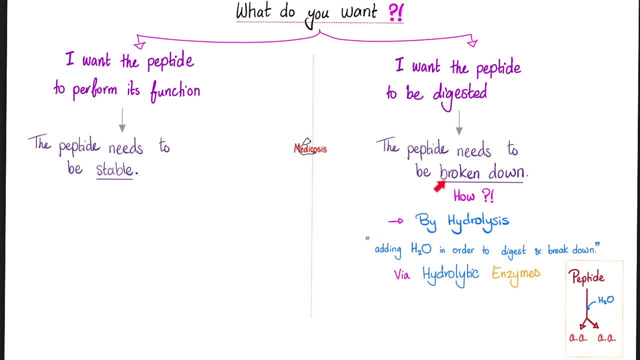 digested, you need to break it down. How do I break down the peptide bond? By hydrolysis. What is hydrolysis To break down and to cleave in the presence of WOTA? In that sense, trypsin and 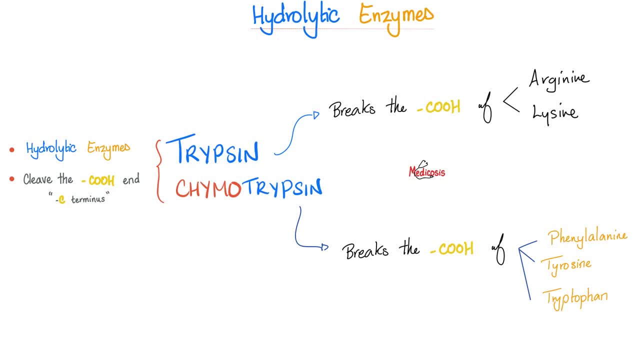 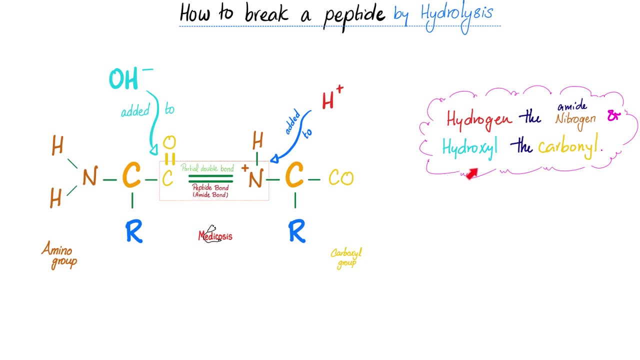 chymotrypsin are hydrolytic enzyme. They cause hydrolysis. They cause hydrolysis, They cause hydrolysis. Look at that. We will add WOTA And this will help us break the peptide bond. Hashtag hydrolysis. Hashtag hydrolase enzyme. So hydrolase means what Ace means: enzyme. And 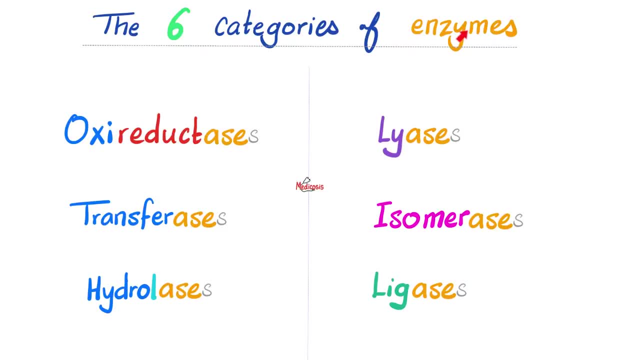 hydro means WOTA. Let's talk about six categories of enzymes. We'll talk about oxyreductases, transferases, hydrolyses, lyase, isomerase and lygase. As you see, all of them end in ace If. 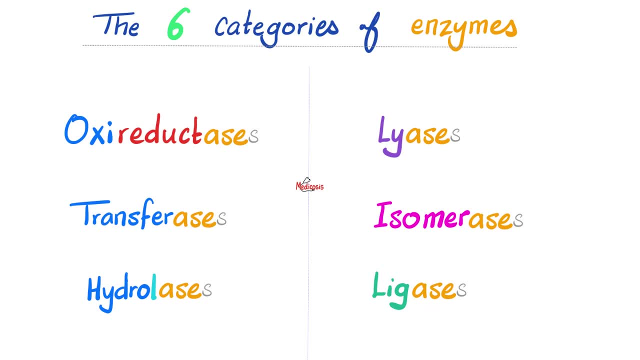 ace on your exam. odds are they are talking about an enzyme. Hey, Medicosus, does the enzyme have to have ace as a suffix? No, it doesn't have to, but it usually does. And here's a pro tip. 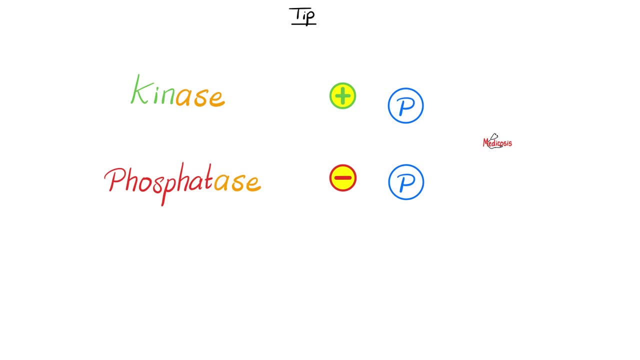 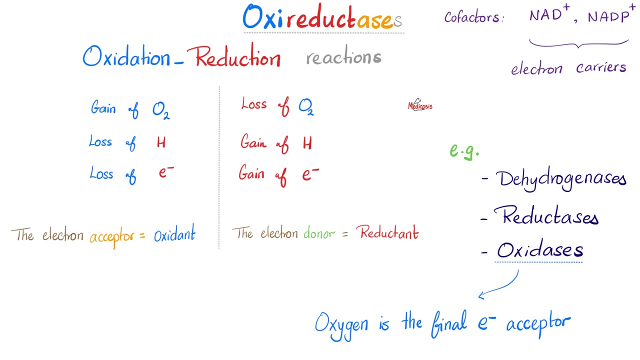 When I say kinase, I mean it's going to add a phosphate. Phosphatase is something to remove the phosphate. Let's start by oxyreductases- enzymes for oxidation reduction reactions. What the flip is oxidation. Oxidation in chemistry could be one of three things. 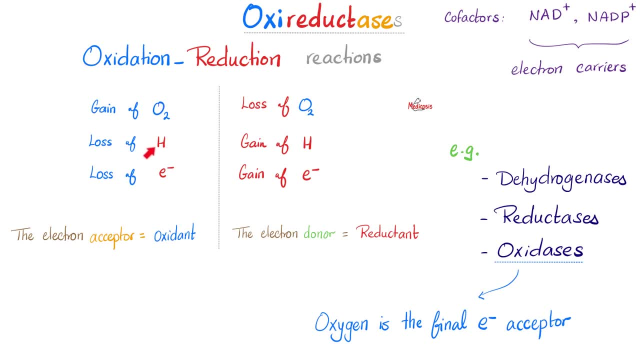 It could be a gain of oxygen oxidation. A loss of hydrogen is also oxidation, A loss of a negative electron. When you lose the negativity, you become a positive thing called oxidation. Conversely, reduction is the exact opposite. Reduction is loss of oxygen, gain of hydrogen. 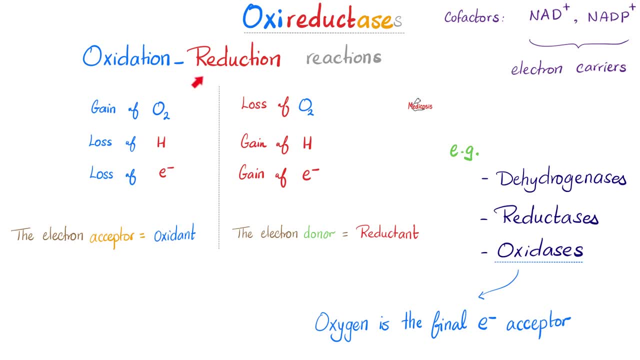 or gain of electron which is negative. In an oxidation reduction reaction, the electron donor is somebody who donates a negative electron. Oh, donating a negative is reduction. Yeah, that's why we call it reductant. Conversely, an electron acceptor is an oxidant, Because when you accept an electron, 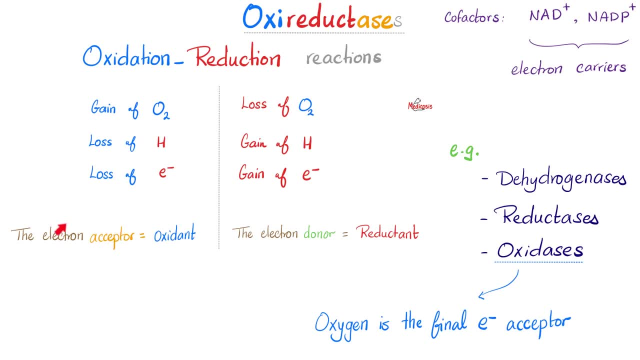 you will take the electron away from the other guy, rendering him oxidized by removing the negativity from him. Oxidation reduction reactions will involve cofactors like NAD and NADP, as we will discuss later in metabolism. Now I want you to remember that the word dehydrogenase, reductase or oxidase means an. 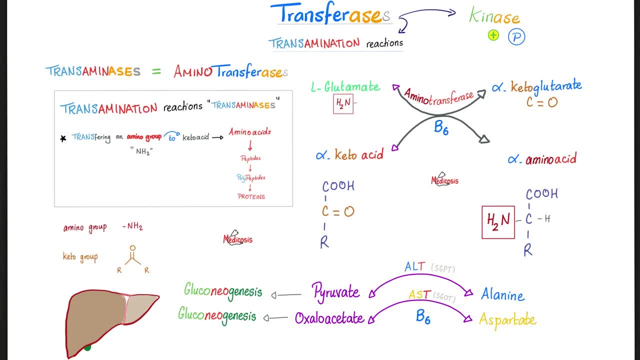 enzyme involved in oxidation reduction reaction After oxy-reductases. let's talk about transferases. If you remember my video about vitamin B6, we talk about transaminase reaction- A transaminase like AST or ALT. this is aspartate aminotransferase and alanine aminotransferase are transferases of. 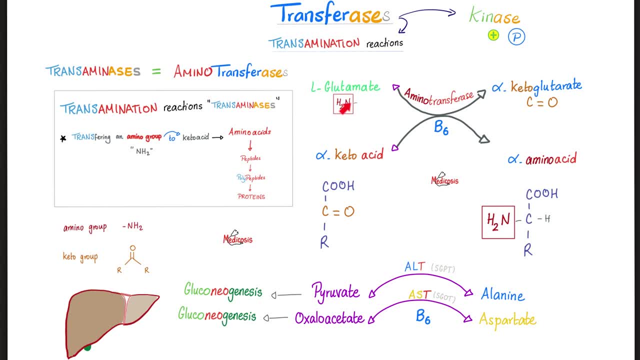 amino And we call them transferases of amino. And we call them transferases of amino And we call them transaminases because they transfer the amino group. For example, if you take that amino group from L-glutamate, the L-glutamate now has lost its amino. L-glutamate will become alpha-ketoglutarate. 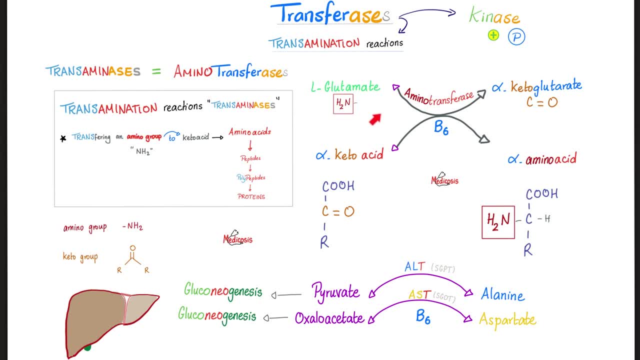 Okay, Metacosis, I took the amino group. Who should I give it? to Give it to the alpha-ketoacid so that it becomes an alpha-aminoacid. Example: ALT will convert alanine to pyruvate. AST will convert aspartate to oxaloacetate. Both. 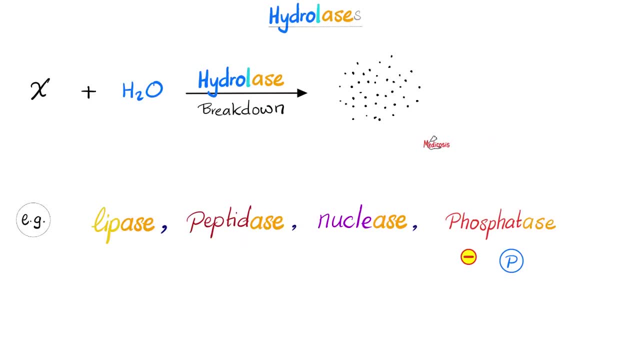 require vitamin B6 as eco-factor. Next, what's a hydrolase? ACE is an enzyme. hydro means water. It's an enzyme that breaks down in the presence of water. Hydrolases could be lipases, peptidases, nucleases or phosphatases. Lipase is an enzyme that breaks down lipid in. 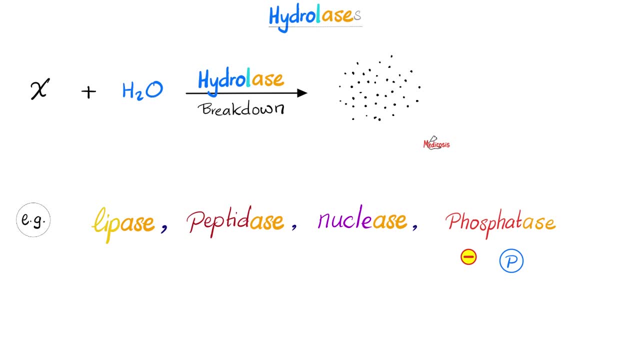 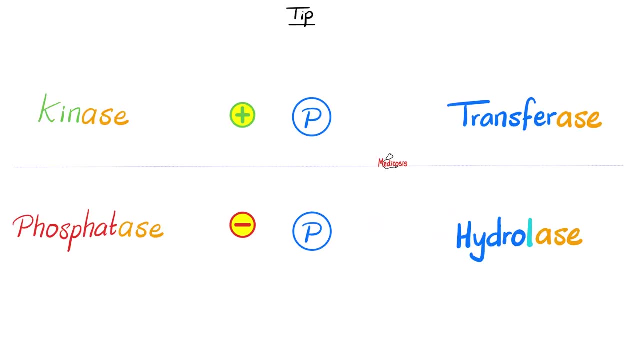 presence of water, Peptidase breaks down peptide. in presence of water, Nuclease breaks down nucleic acid. Phosphatase breaks down phosphate. So I hope you realize that kinases add phosphate and they are examples of transferases. They 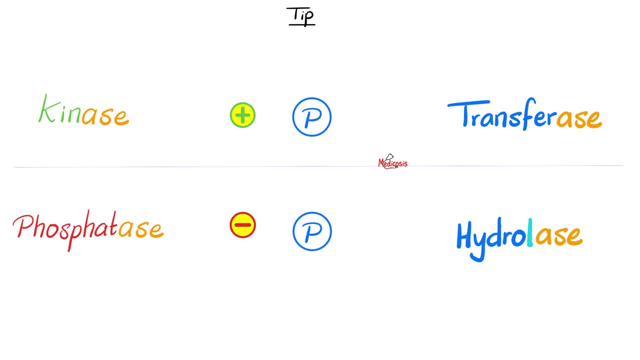 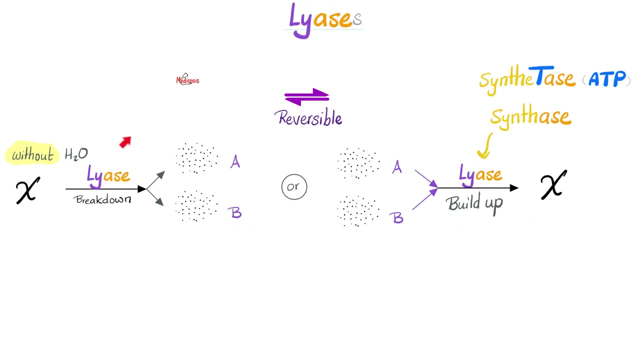 transfer a phosphate group to you, They give you a phosphate. That's a transferase. Conversely, phosphatase, which removes a phosphate, is a hydrolase. It breaks down your phosphate. It takes the phosphate away from you in the presence of water. What's a lyase then? A lyase is something. 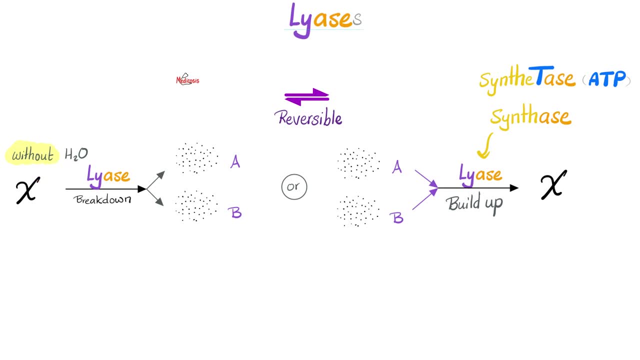 that breaks down. but in the absence of water, Unlike the hydrolase, lyase goes both ways. So I can break down X into A and B, or I can bind A and B together to give you X again. Lyase goes both ways. It's a reversible reaction. Oh, by the way, 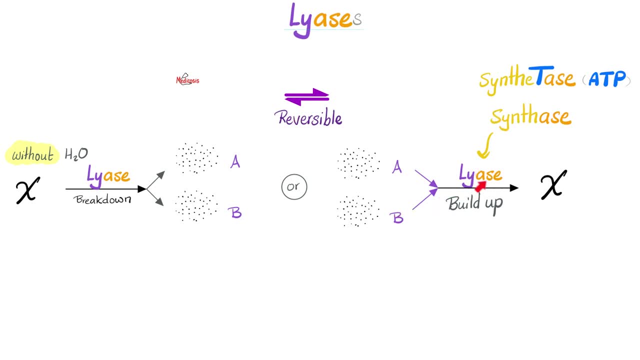 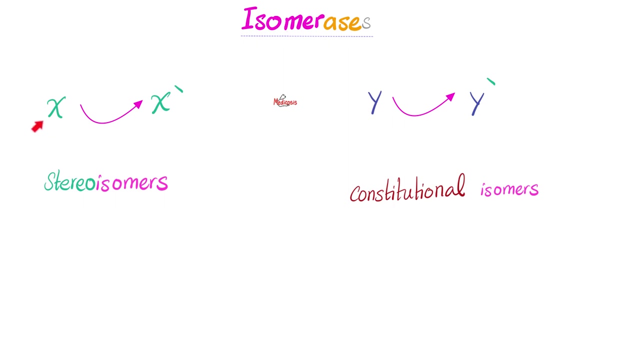 when I use lyase to build up here, you can call it something else, You can call it synthase, And if you need ATP for the reaction, we can call it synthetase. What's an isomerase? It's an enzyme that will convert you to your isomer. Could be a stereoisomer. 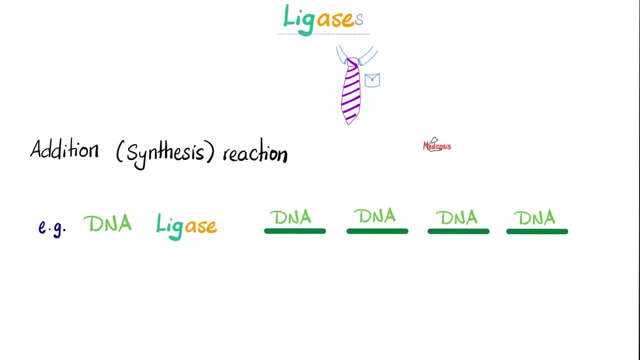 or a constitutional isomer. What's a ligase then? It's an enzyme that ligates. To ligate is to tie. For example, here is a DNA fragment, another DNA, or who's gonna bind them together and tie them together to make a singular long strand ligase. And these are the six categories of enzymes that we see in the adenosine triphosphate. What's an isomerase? It's an enzyme that will convert you to your isomerase. What's an isomerase? It's an enzyme that will convert you to your isomerase. I know this.